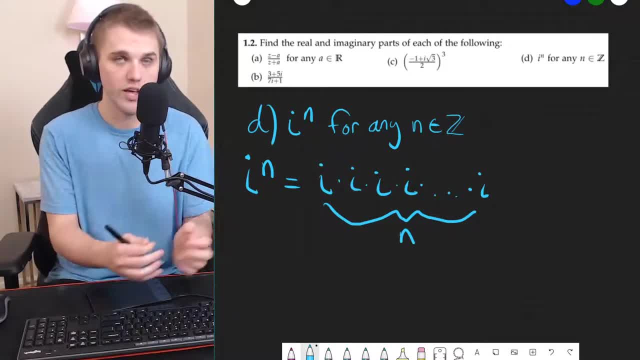 Now this doesn't really help me figure out what the real and imaginary part is, because I would have to multiply all of these i's together to figure that out, And I don't really know how to do that, considering I don't know how many i's I have here. 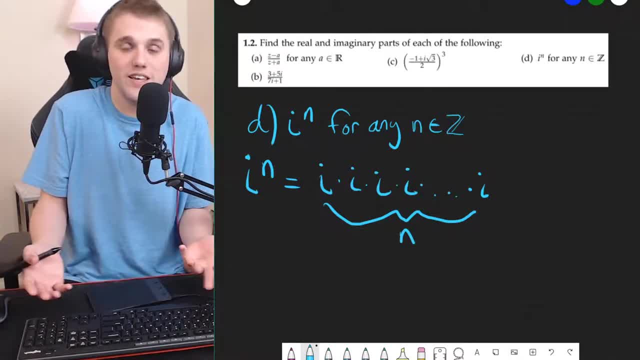 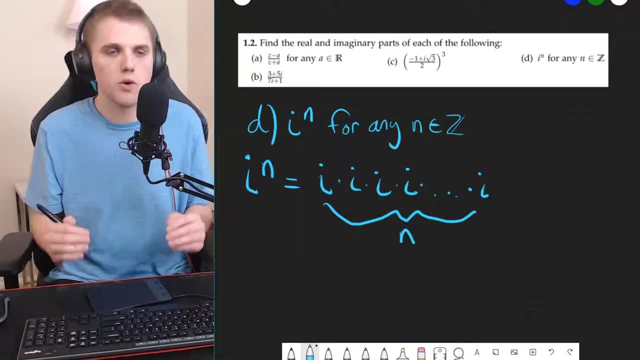 I have n i's, But how many i's is that? It's n? What is n? Some integer, I guess. So here's what we're going to do to try to address this. We're going to pick values of n specific integers for n, and we're just going to look at what i raised to that power is. 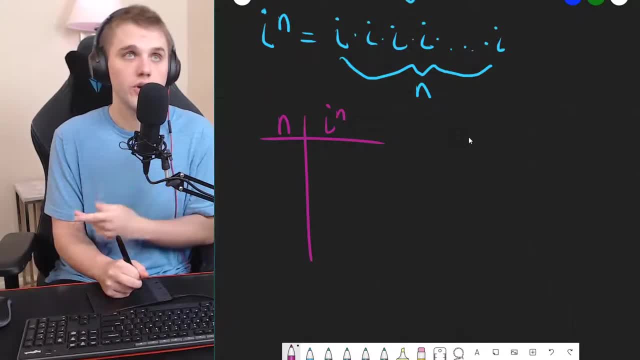 So let's start with a table. So here in the left column I'm going to pick some integers for n. In the right column we're going to try to figure out what i raised to that power is in terms of its real and imaginary parts. 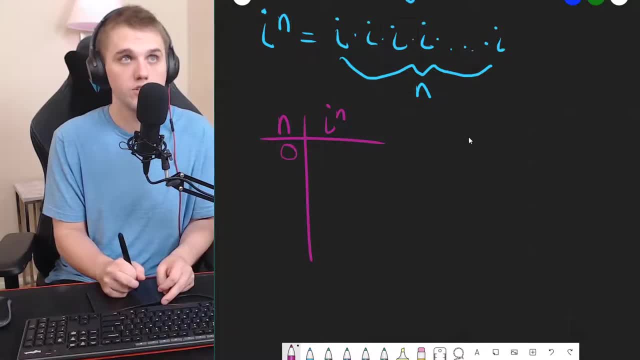 So let's start with some easy n values: 0.. What is i to the 0th power? Well, anything raised to the 0th power, any complex number raised to the 0th power, is 1.. What about when n equals 1?? 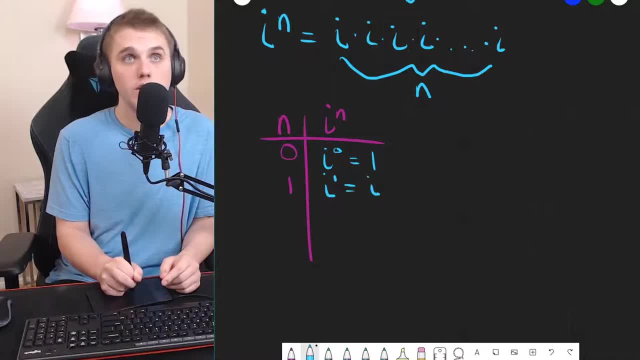 Well, i to the 1th power is i. So here we have a real part that is 1.. And an imaginary part that is 0. When n equals 1, we have a real part of 0. And an imaginary part of 1.. 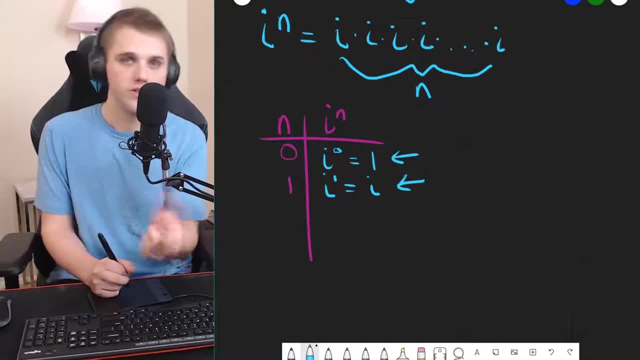 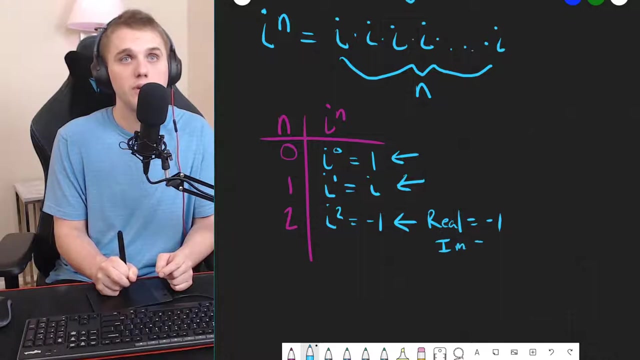 Sort of swapped there. When n equals 2, we have i squared Which is negative 1.. Here the real part is negative 1. And the imaginary part is 0. And then, if we go to 3, we have a real part of 0.. 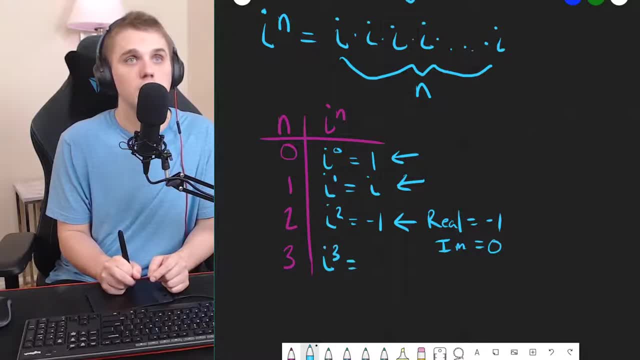 And then if we go to 3, i cubed is just: i squared times i. And if I write it like this, it makes it easy to figure out what i squared times i is, because I already know what i squared is. i squared is negative 1.. 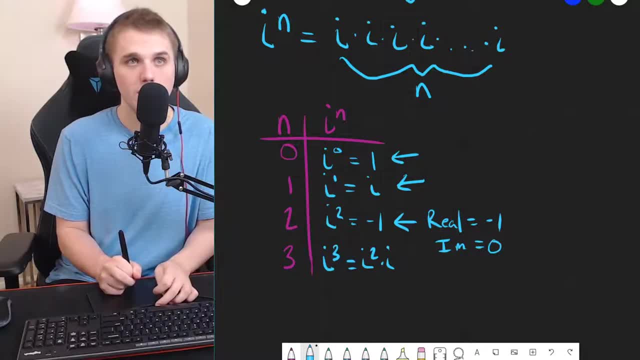 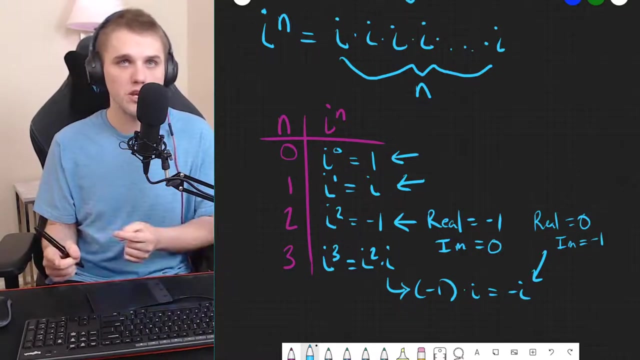 And so i squared times i is negative 1 times i, Which is just negative i, And so in this specific instance, the real part is 0.. And the imaginary part is negative 1.. So you might notice we're rotating between real and imaginary. 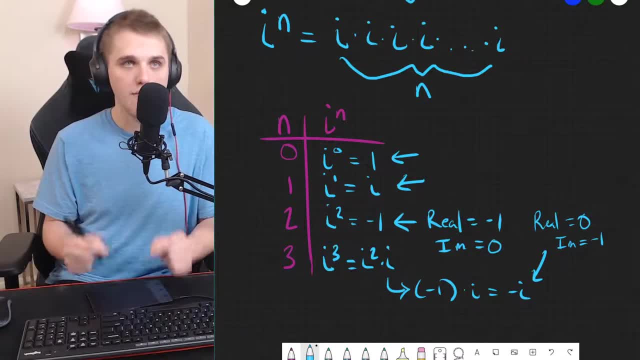 0, 1,, 0,, 1.. And on top of that the signs are flipping. It went from positive to negative. Let's see what happens at n equals 4.. I'm going to give myself some more room here. 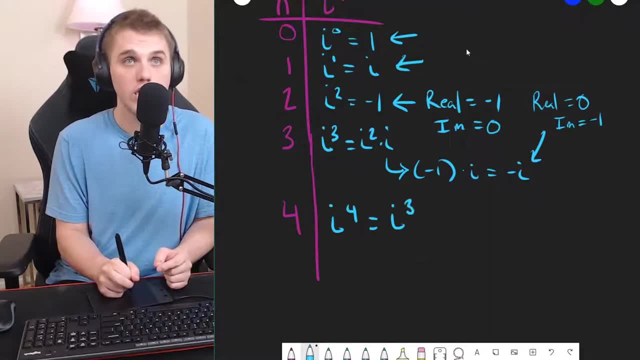 Well, i to the 4th is just: i cubed times i, And I can always do this because then I can just take the result from above and replace that with i cubed here, And I can just keep doing that with whatever number I have minus 1.. 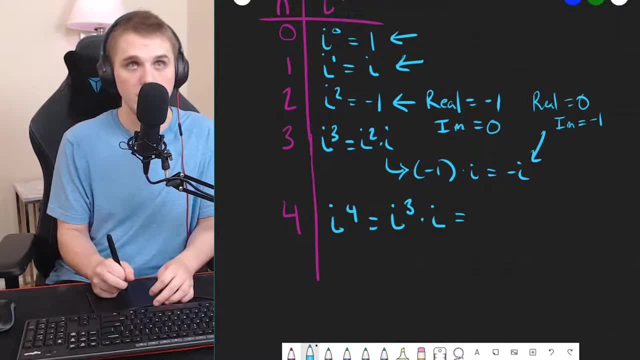 I can just replace with the above result and rinse and repeat. So this is negative i times i, Which from here we can see is negative i squared And negative i squared is negative, negative 1.. Which is just 1.. i squared is negative 1.. 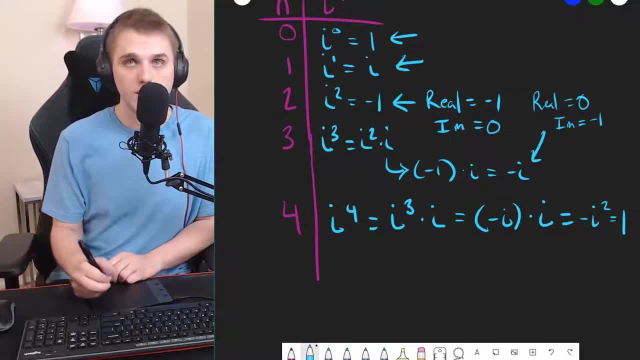 So negative, i squared is positive, 1.. So in this instance the real part is 1. And the imaginary part is 0.. Which is the same as this instance here, Where the real part is 1. And the imaginary part is 0.. 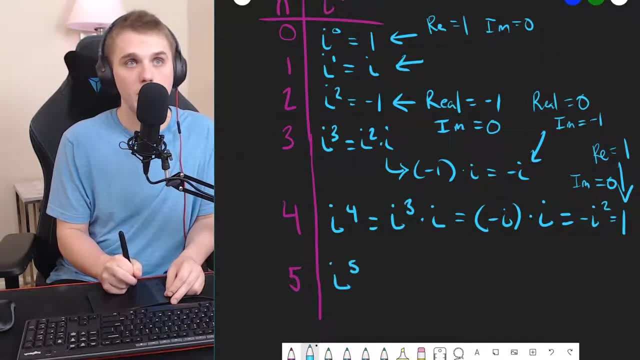 Let's go to n equals 5.. Here i to the 5th power is just i to the 4th power times i. And we do this so that we can take the result from our previous output And we can say: this is 1 times i. 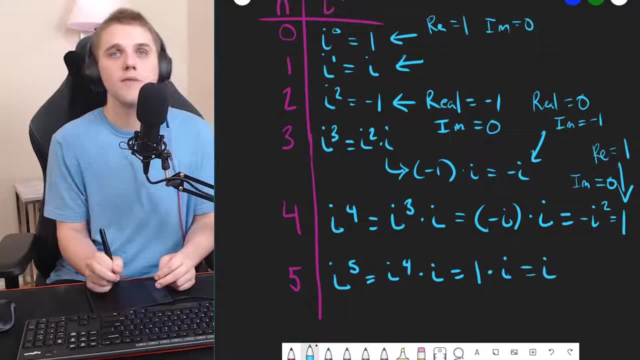 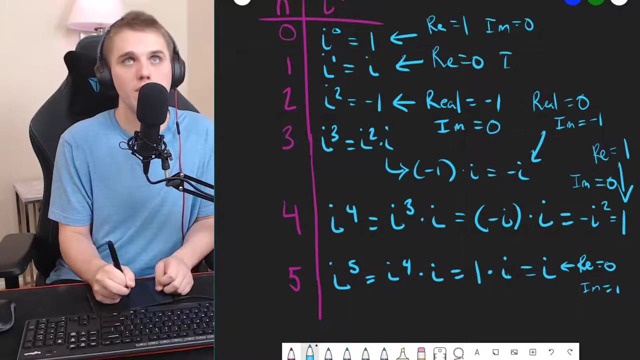 Substitution, Which is just i, And in this instance we have the real part is 0. And the imaginary part is 1.. Just like above, we had a real part here was 0. And the imaginary part was 1.. 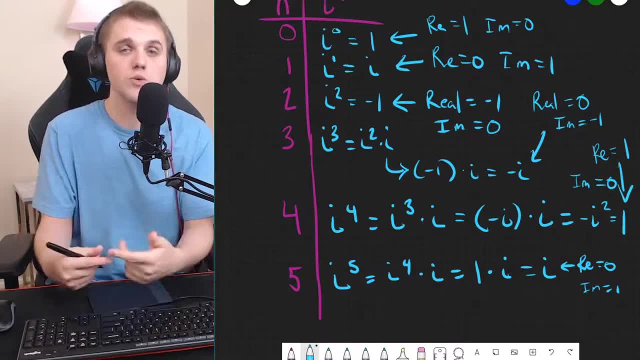 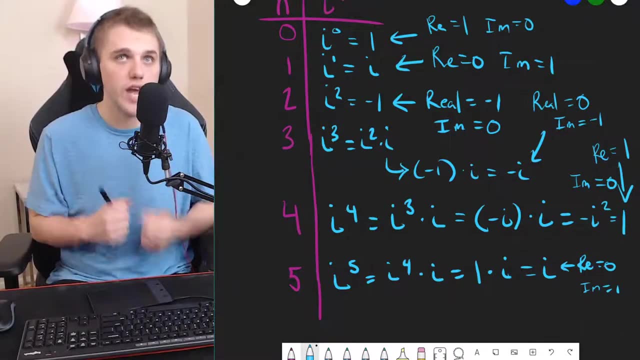 And so you might notice that we're going into a cycle. We're just going back and forth here, We're alternating, So it's 0, 1, 0, negative, 1, 0, 1, 0, negative 1, 0, 1.. 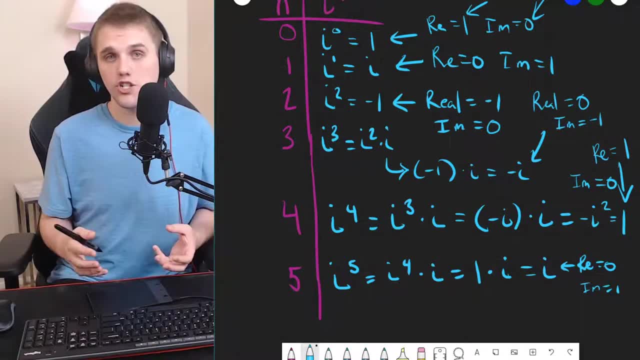 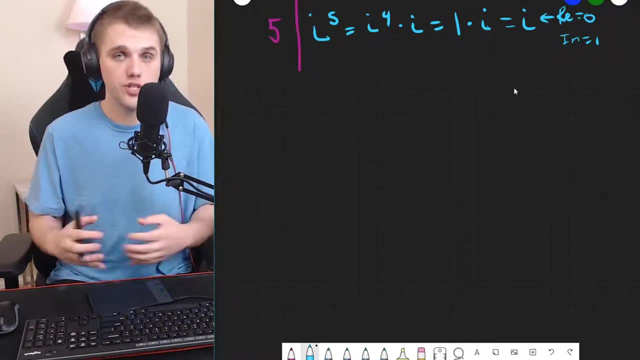 So let's try to represent this relationship with some formula Now in complex analysis. technically I haven't introduced the divides operation, Although I have done videos on the divides operation And I highly recommend you take a look at those. 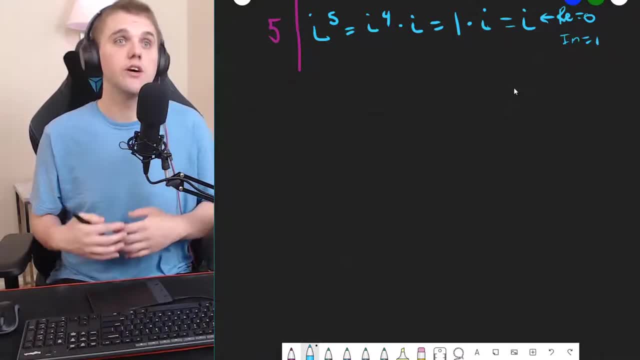 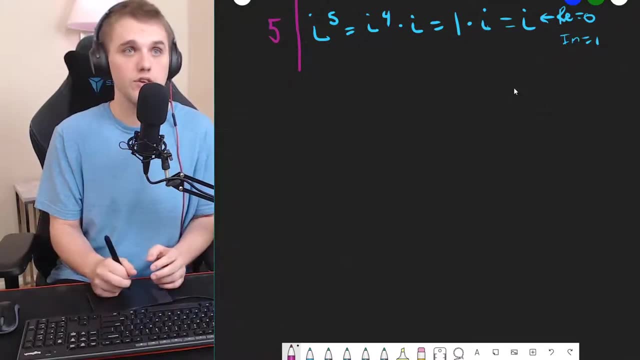 I'm going to try to make this function definition a little bit more approachable, So this might look a little sloppy, But bear in mind, I'm doing this so that everyone can understand what i to the n is. i to the n is one of four things. 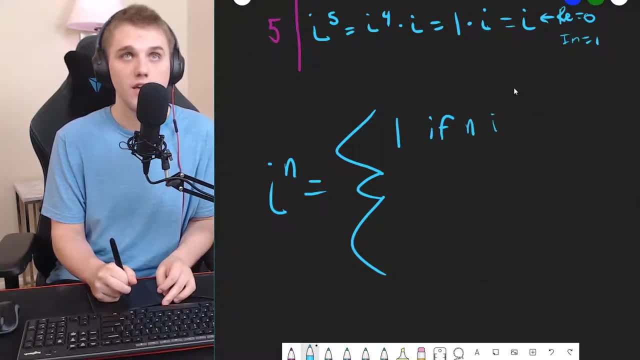 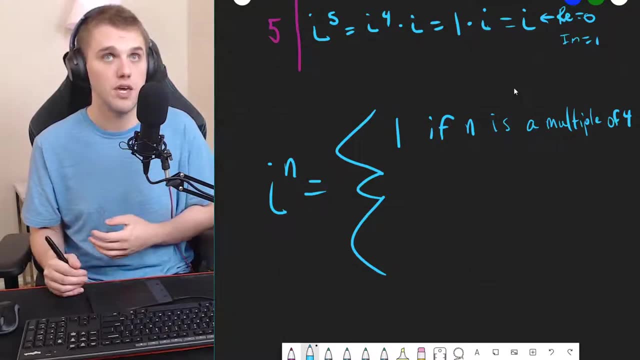 i to the n is 1.. If n is 0. i to the n is a multiple of 4.. Now I should clarify. When I say multiple, I mean it could be 4 or 8 or 12 or 16.. 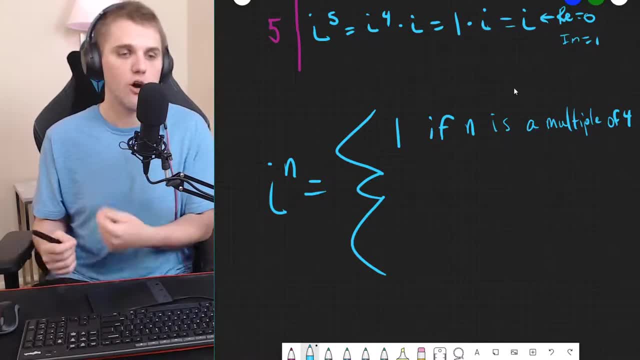 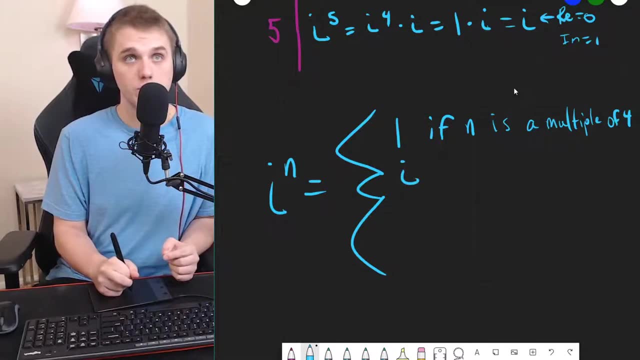 Or even 0 or negative 4 or negative 8.. Specifically, all of the integer multiples of 4.. And then for n equals 1, we get i as a result. But that is when n equals 1 or n equals 5.. 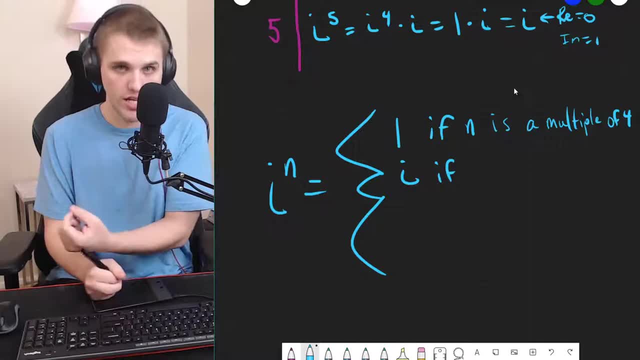 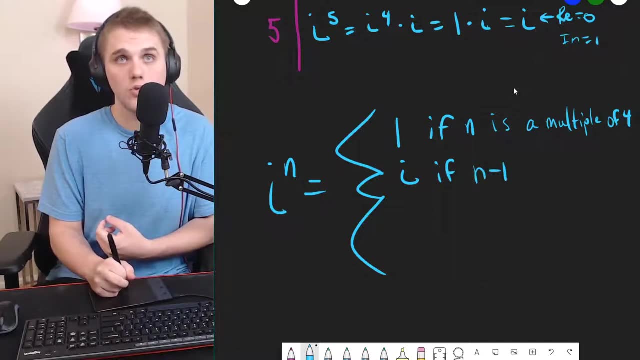 Or n equals 9. Or n equals 13.. So how do we represent those numbers? Well, if we just take that number and we subtract 1., Then we're back to a multiple of 4.. So is a multiple of 4.. 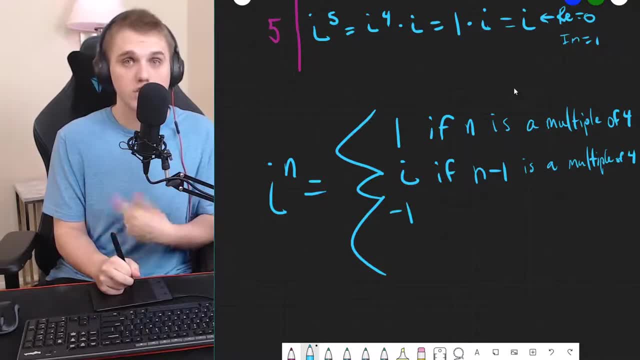 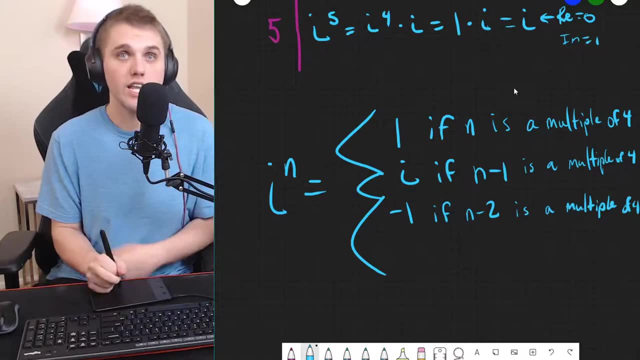 And then up next we have negative 1. Because i squared is negative 1. If n minus 2 is a multiple of 4.. Again, technically, this portion is a concept that I developed In my number theory lectures, My number theory videos. 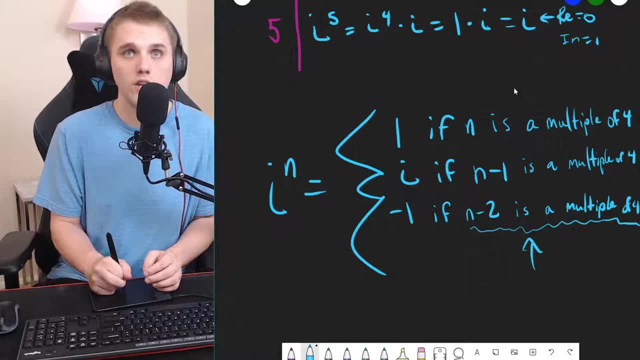 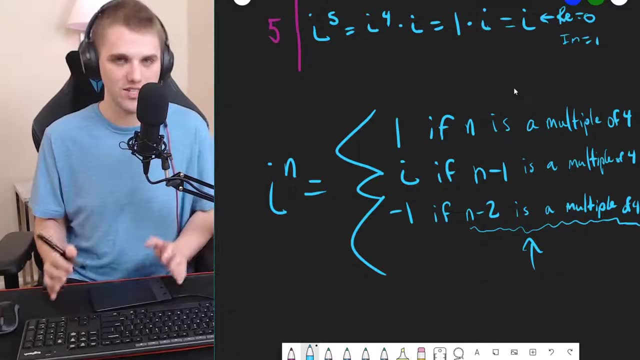 And so I don't expect you to understand how we developed this portion. So if I were to make a test for my complex analysis students, I would not ask this question explicitly, Because this requires a little bit of number theory to understand. 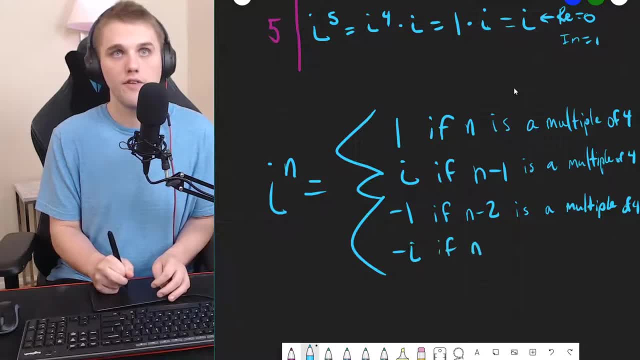 And then, lastly, we have negative i. If n minus 3 is a multiple of 4. And I'll just put quotation marks just to represent, It's the same as above. So we're not done yet. I want to identify what the real and the imaginary part of i to the n is.